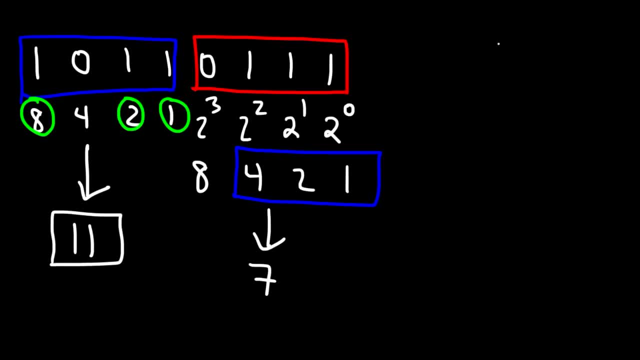 Now we need to convert these numbers into the hexadecimal values. Ten corresponds to A and eleven corresponds to B. So we're going to replace eleven with B. We have B7, B16.. So the binary number 10110111 correlates to this in the hexadecimal system. 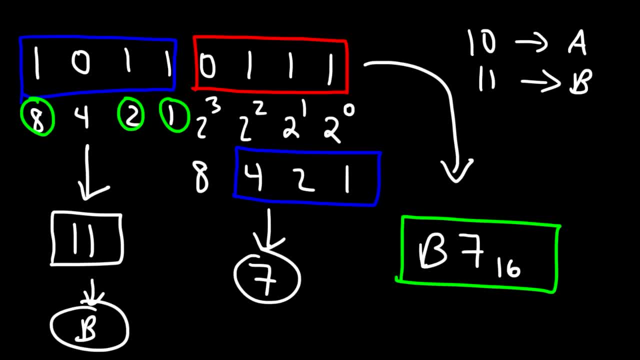 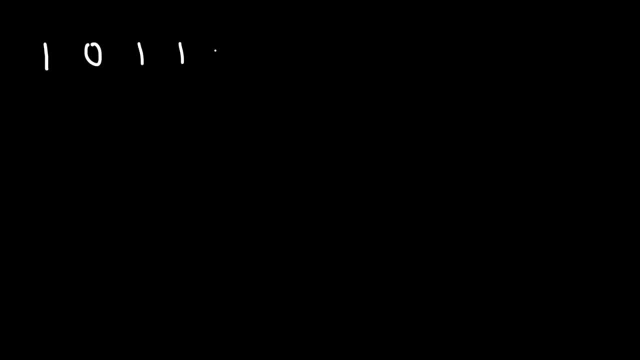 And so that's how you can convert a binary number into a hexadecimal number. Now for the next example. let's say it's 101110.. Go ahead and convert this binary number into a hexadecimal number. So, like before, let's break it up into groups of four. 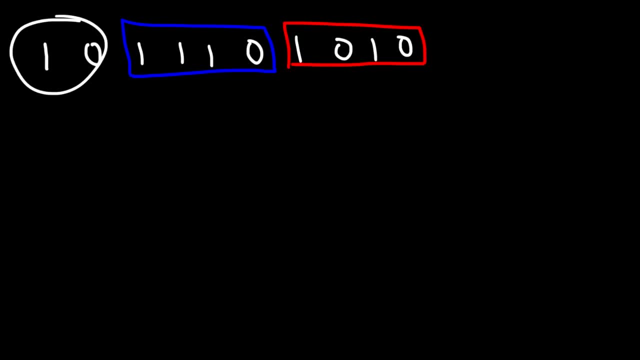 Now notice that we don't have four numbers here, so we can add two zeros. So the first group will be 0010, and then the second group will be 1110.. And the last one is 1110.. So let's start with the first group. 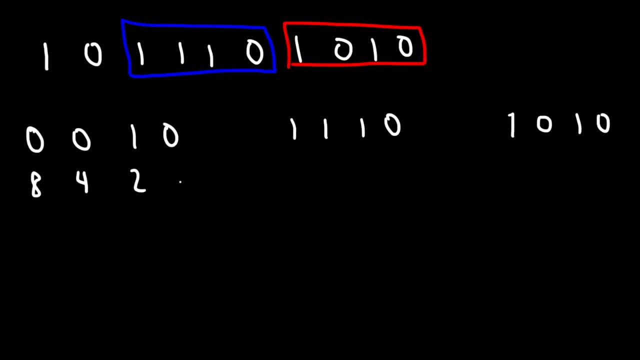 So we have the numbers eight, four, two and one. So we only have a value of two here. For the zeros, just ignore them. So this number- 0010, corresponds to a value of two. For the second group of four, we need to add two zeros. 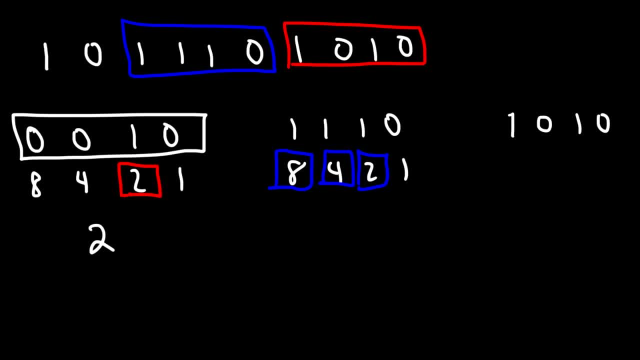 We need to add eight plus four plus two. Eight plus two is 10,, 10 plus four is 14.. And for the last one, the significant values are eight and two, which will give us 10.. Now recall that 10 corresponds to A, 11 corresponds to B, 12 corresponds to C, 13 corresponds to D. 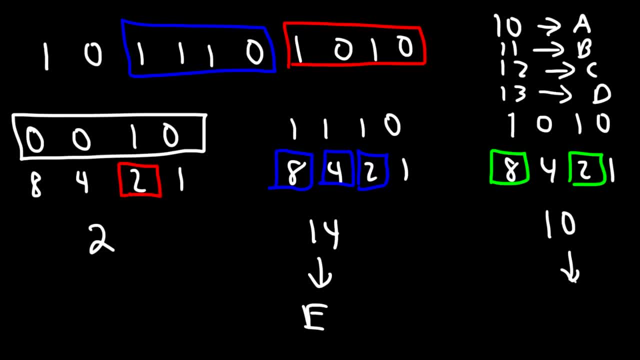 which means 14 corresponds to E. We could replace 10 with A, So the answer is going to be 2EA. So it's 2EA in the hexadecimal system, And so that's it. That's how we can convert this binary number into a hexadecimal number. 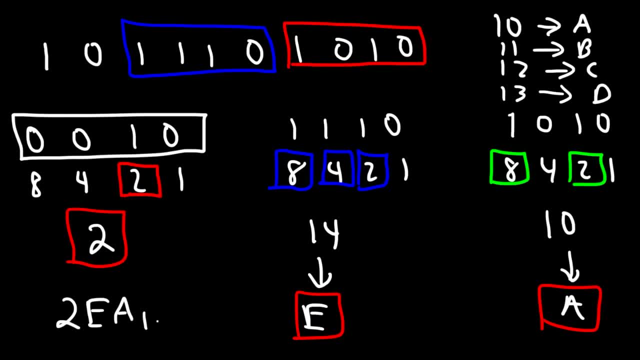 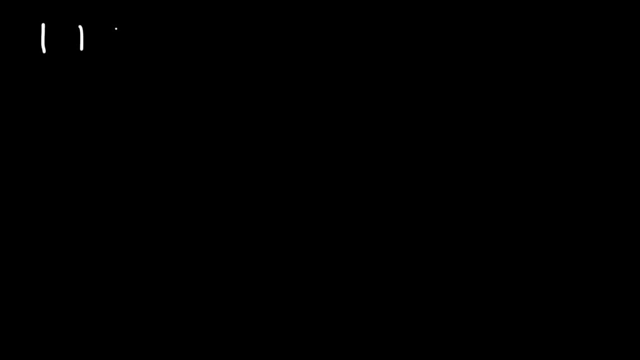 Now let's try another example: 1, 1, 1, 1, 0, 1, 1, 1, 1, 1, 1, 0, 0.. Try that one. 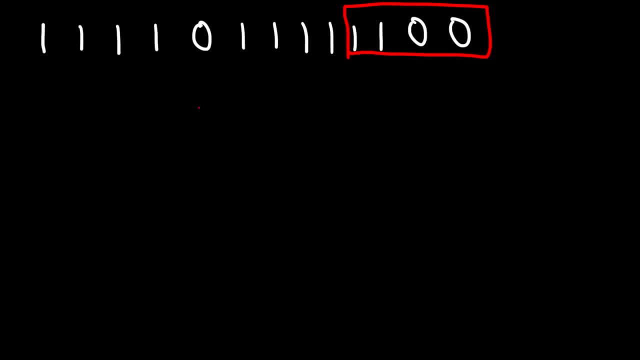 So let's separate it into groups of four. So the first group: we're going to add three zeros, So it's going to be 0, 0,, 0, 1.. And then the group in green is 1, 1, 1, 0.. 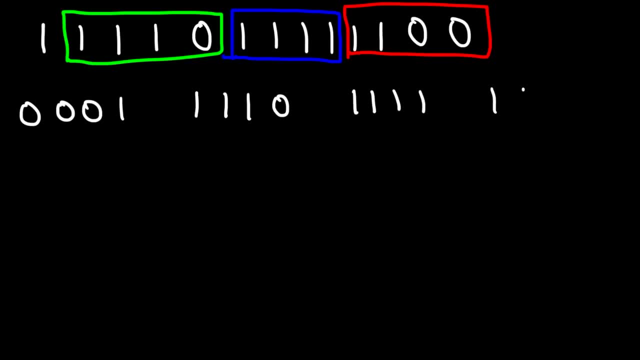 And then in blue 1, 1, 1, 1.. And in red 1, 1, 0, 0.. So for this one, only this number is significant. So we have two zeros, We have a value of 1.. 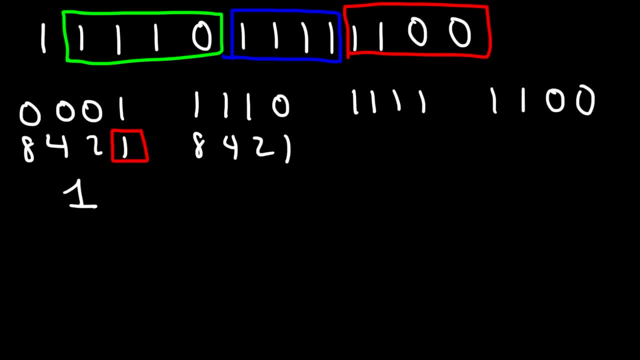 For the second one, the numbers 8,, 4, and 2 are important, So 8 plus 4 plus 2, that's 14.. And for the last one, all of them are important, So they add up to 8 plus 4 plus 2 plus 1, that's 15.. 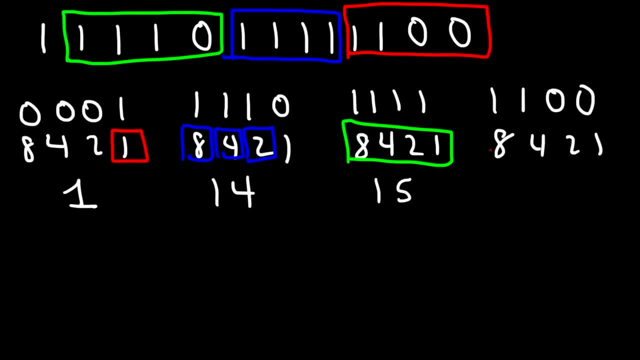 And for the final one it's just 8 plus 4, which is 12.. So we know: 10 is A, 11 is B, 12 is C, 13 is D, 14 is E, 15 is F. 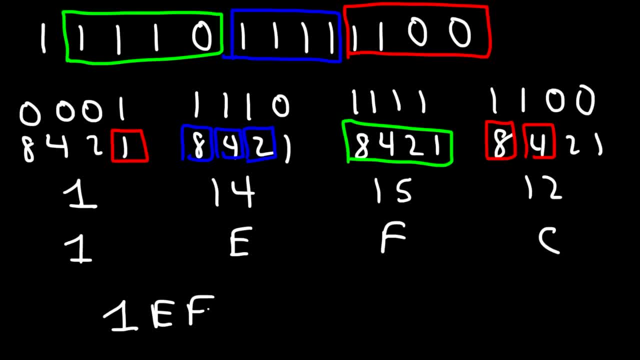 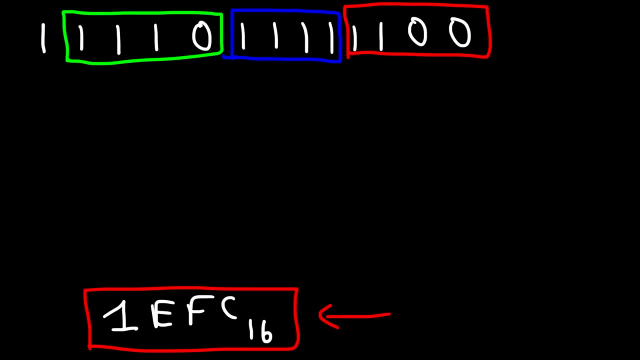 And so the answer is 1, E, F, C And then the base 16 system. So this is our answer as a hexadecimal. Now, to make sure that we have the right answer, let's convert the binary number and the hexadecimal number. 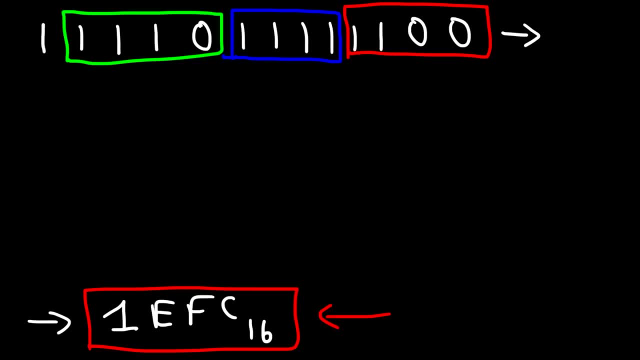 into a decimal value And let's make sure that it's the same. So let's start with the binary number. So this is 2 to the 0,, 2 to the first, 2 squared 2 to the third, fourth, fifth, sixth and so forth. 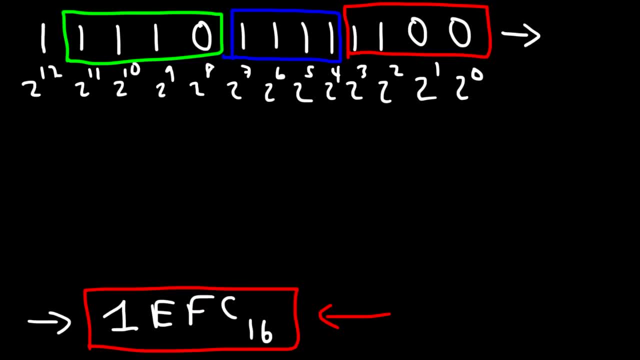 So we have a 1 associated with 2 to the 12th. So 1 times 2 to the 12th, that's going to be 4,096.. And then we have 2 to the 11th, which is 2,048.. 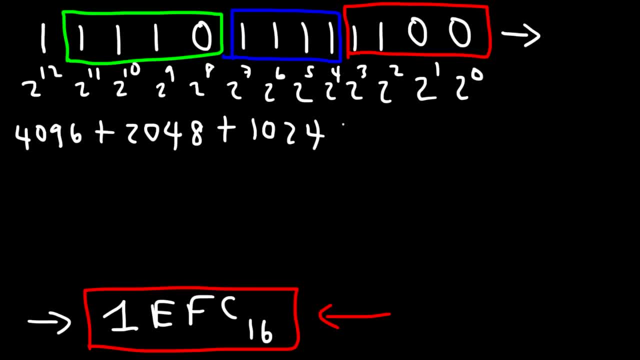 And then 2 to the 10th, which is 1,024.. And 2 to the 9th, which is 512.. And then 2 to the 7th, that's 128.. 2 to the 6th is 64.. 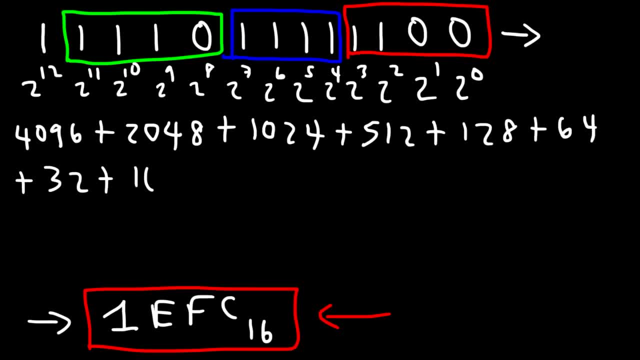 And then 2 to the 5th, which is 32.. And then we have a 16,, 8, and a 4,, which is the last one, 2 squared. So if we add up these numbers, 4,096 plus 2,048,. 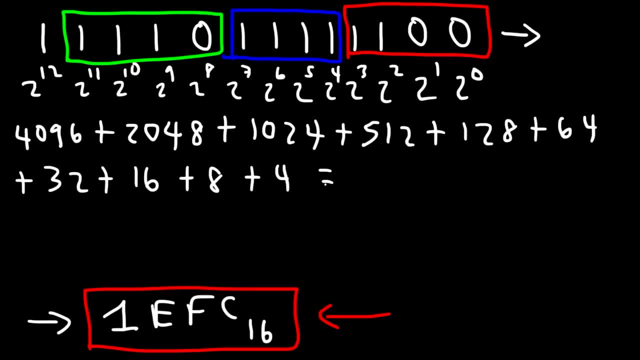 plus 1024,, plus 512, plus 128n, all the way to 4.. This will give us 7,932.. So now let's convert the hexadecimal number into a decimal number. Let's see if we get the same thing. 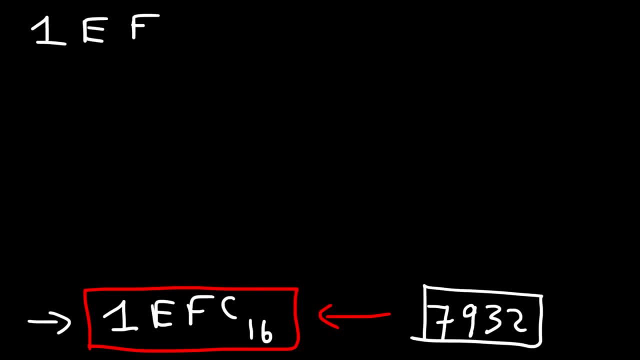 So we have 1EFC. So we know E corresponds to 15. And E corresponds to 14.. F corresponds to 15. And C corresponds to 12.. We need to multiply C by 16 to the 0 power. 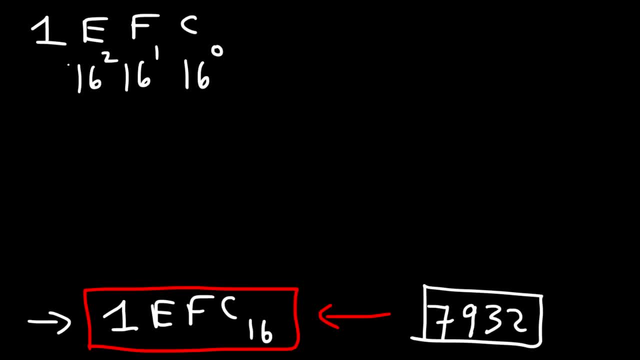 F by 16 to the 1st, E by 16 squared And 1 by 16 cubed. So it's 1 times 16 cubed And we said E corresponds to 14.. So it's going to be plus 14 times 16 squared.